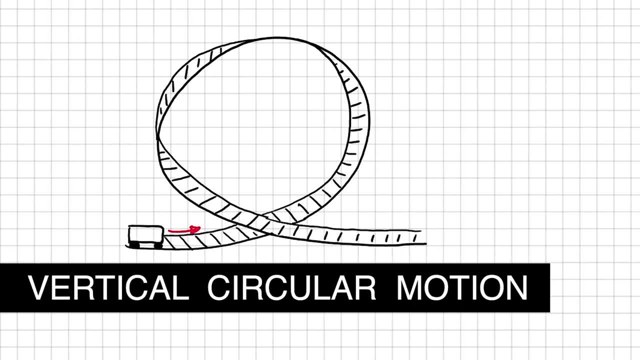 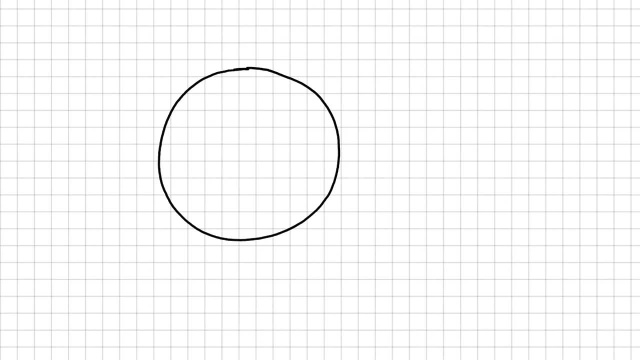 A roller coaster goes down the track and loops the loop in a vertical circular motion. We are making the approximation that this circular motion is a perfect circle. What are the forces providing the centripetal force making it follow this curved path, And are they going to be the same whether the roller coaster car is at the bottom of the loop? 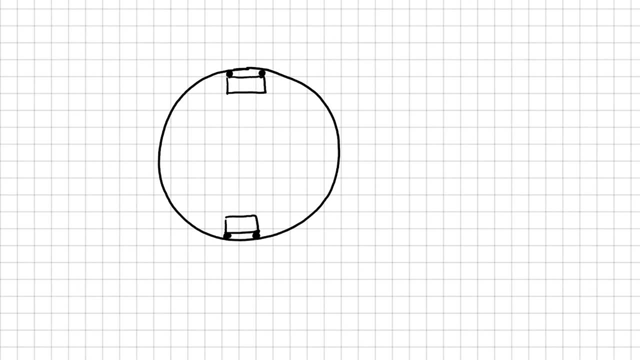 or at the top. Let's find out starting with the car. at the lowest points in this vertical circular path, Centripetal force always acts towards the center of the circular path And the centripetal force is given by the equation mv squared over r, where m is the mass of the. 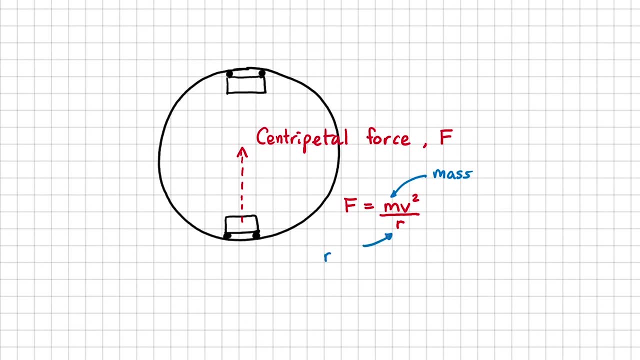 object traveling in a circular motion with a radius r, The object's tangential speed is v. When the car is in this position, the weight of the car is acting downwards, but normal reaction force from the roller coaster track is acting upwards. and I'm going to rewrite. 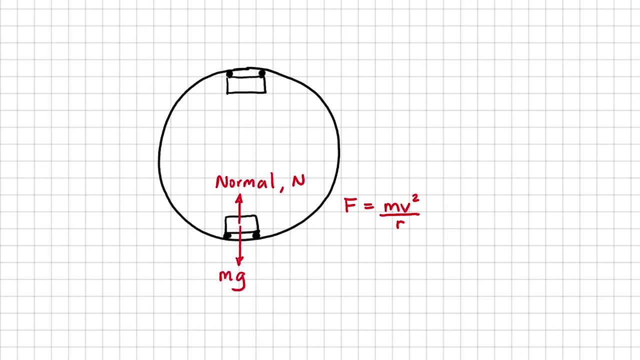 the weight of the car as v, weights of this object as mass times, gravitational acceleration, mg. So I'm going to equate the centripetal force to the normal reaction force which is pointing towards the center. but since mg is acting away from the center, I'll put a minus sign in front of it When the car is at the top. 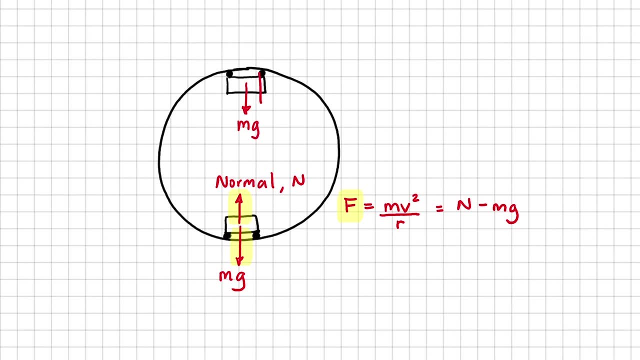 the weight, or mg, is still acting downwards and the normal reaction force is also acting towards the center. So I need to set up my equation like this: Centripetal force is equal to the normal reaction force plus mg. Let's look at another vertical circle of motion scenario. 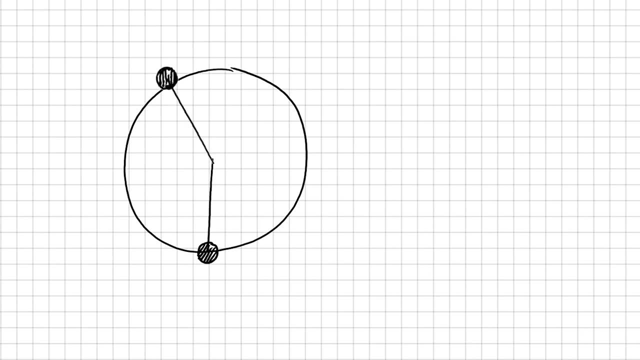 I'm swinging a ball around vertically at a constant speed by keeping the centripetal force constant. What do you think will happen to the tension in the string when the ball is at different positions? At the bottom, tension in the string is acting towards the center, but mg is acting. 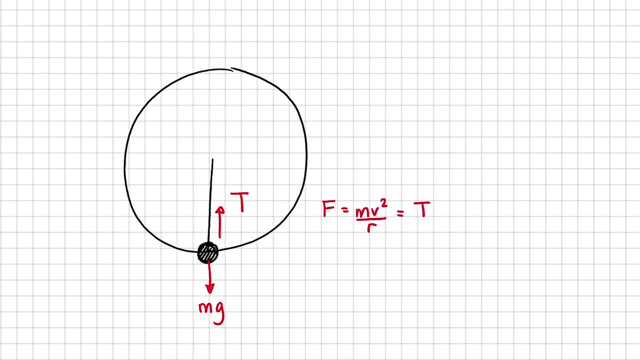 downwards. So I need to set up my equation like this: Centripetal force is equal to the normal reaction force plus mg. I'll rearrange this to make tension the subject. When the ball is at the top, tension is still acting towards the center of the vertical circle of motion, and this time